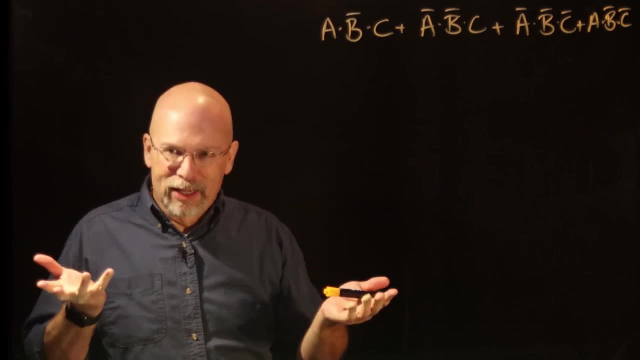 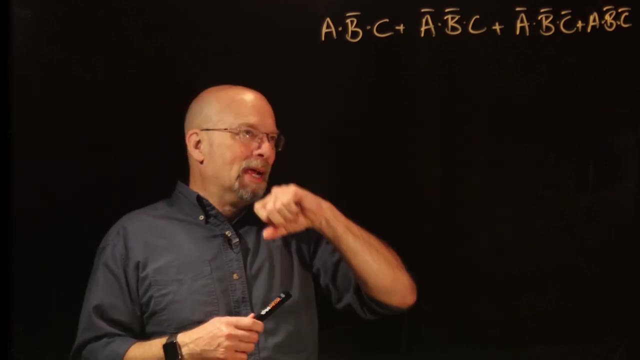 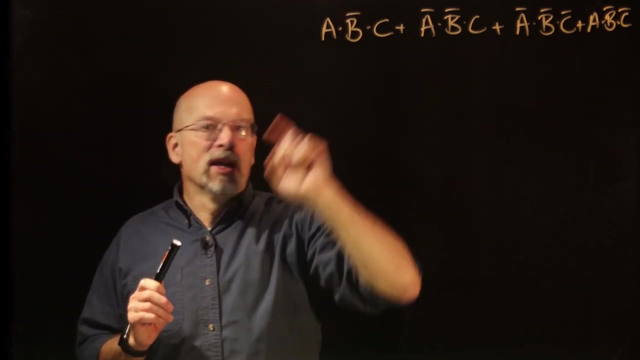 its inverse, or something's being combined with a constant, The only constants we have available to us: zero and one, So I don't see it. I don't see anything right away. What we can see, though, is that b bar is in every single one of those products, So we can use the standard form of the distributive. 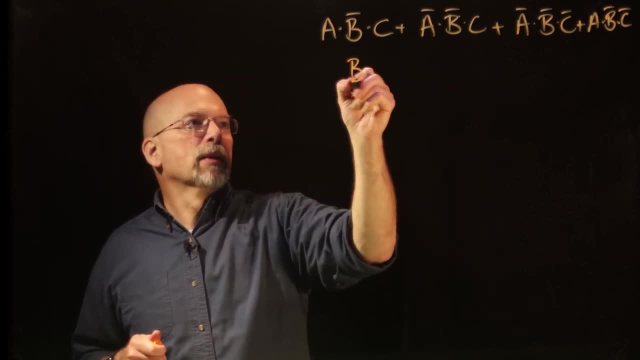 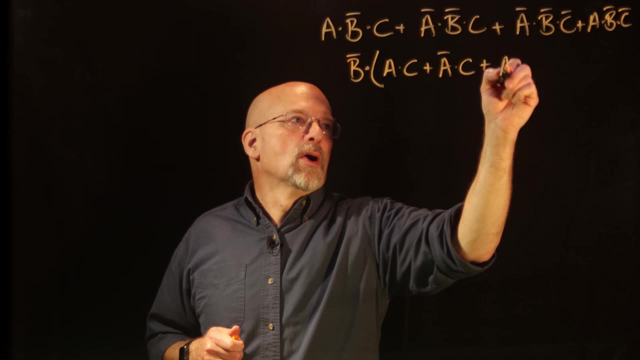 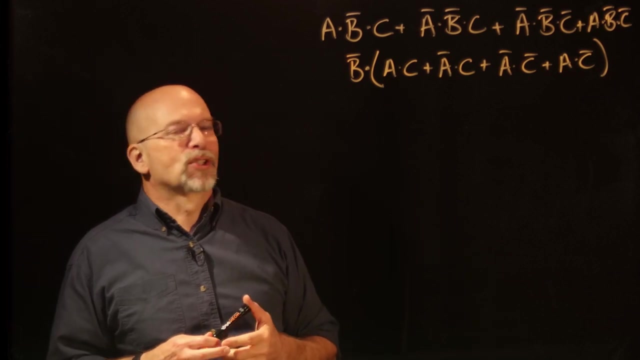 law to pull out a- b bar. So I can pull out b bar anded with a and c, or a bar and c, or a bar and c bar, or a bar and c bar. Okay, still no red flags. Well, what else could we massage around? What else could we? 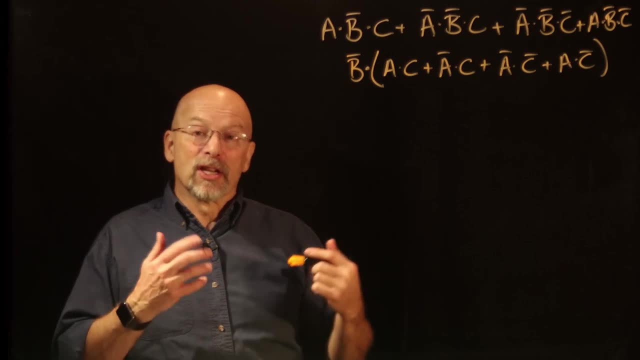 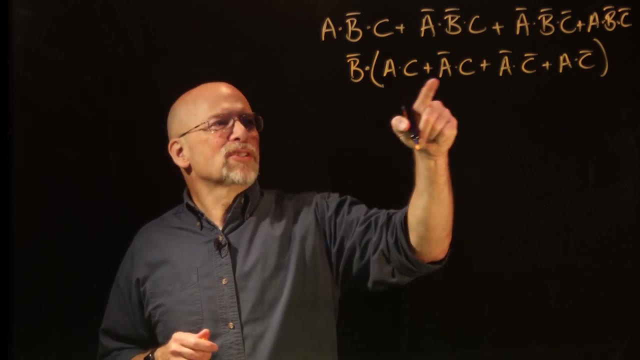 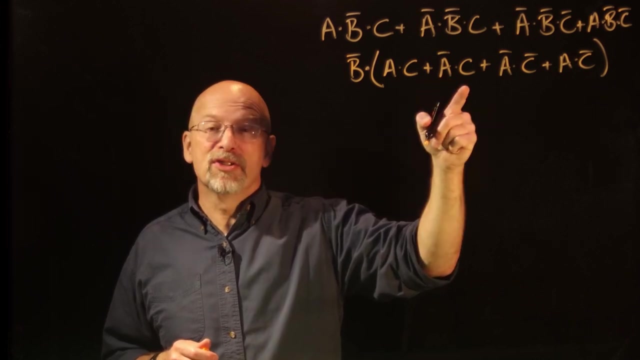 move around when it comes to this expression, to make it so that it's possibly a little well. so something shows up that we can simplify. Well, if you see these first two terms, they have one, has a, one has a bar. They both have c. If we pull c out, we can see that. 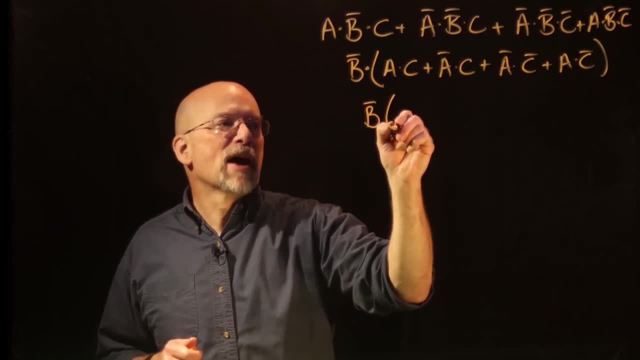 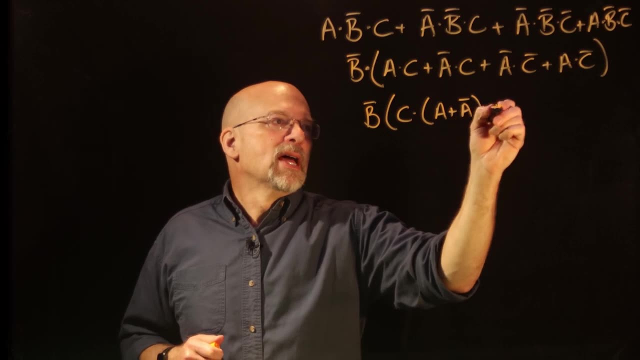 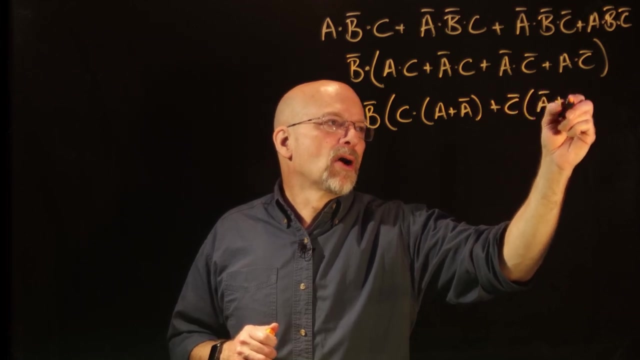 c, a or a bar. Let's go ahead and do that for those first two terms, So kind of embedding these parentheses a or a bar, And then we can do a similar thing for this last term. I can pull out c bar and have a bar or a Now, and in fact you know we've talked about 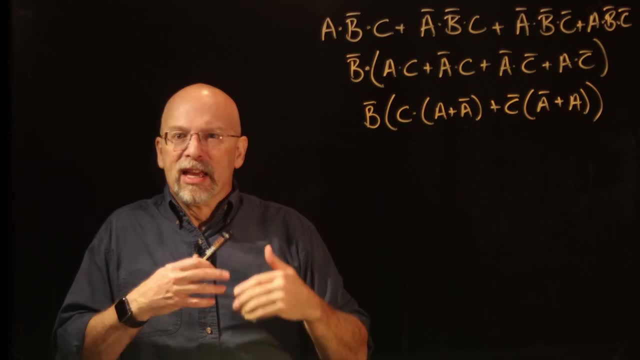 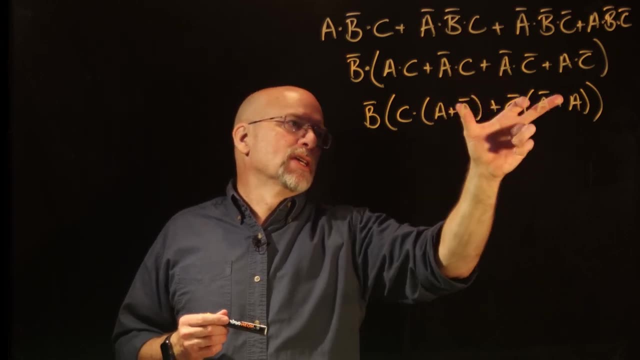 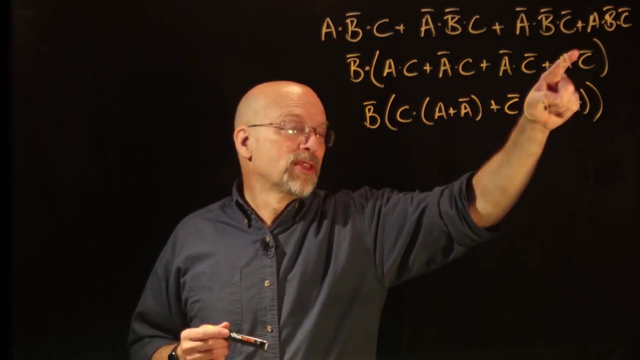 this before, where there's usually more than one path to reach a final simplification, If I had swapped these two terms. now let's see if I had swapped these two terms through the commutative law, so the this product swapped with this product instead of pulling. 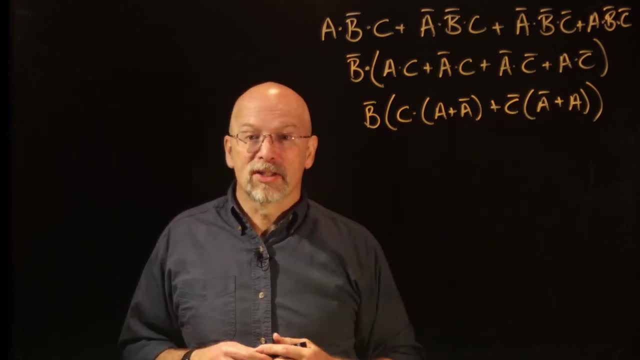 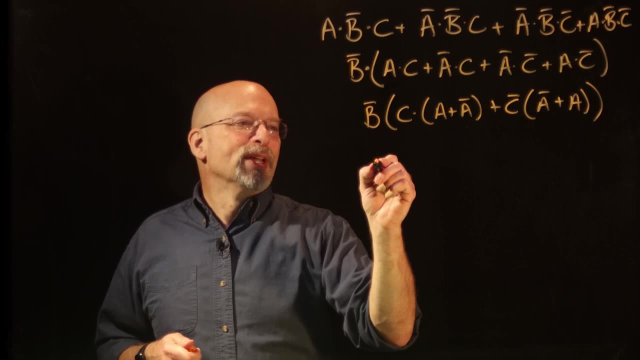 c out. I could have pulled a out of the first two terms and a bar out of the second two terms. So, really, the path we're taking just happens to be the path we're taking Now. we do have a red bar- excuse me, a red flag- showing up, don't we? We have something, orred. with its inverse and something orred with its inverse. Okay, so we have something orred with its inverse and something orred with its inverse. Okay, so we have something orred with its inverse and something orred with its inverse. 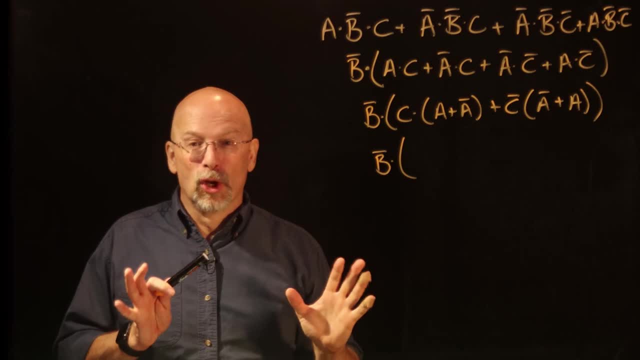 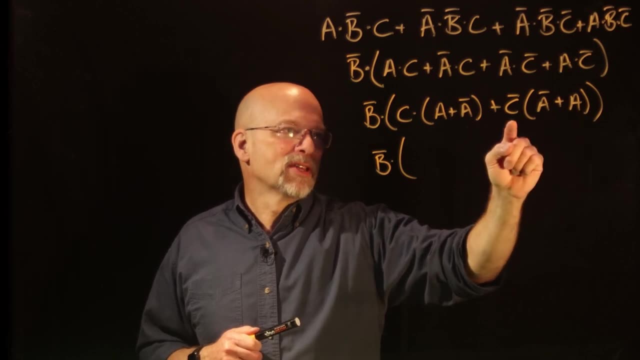 Okay, so we have something orred with its inverse and something orred with its inverse. with its inverse, Turns out it's the same thing. There's, in fact, two ways we could do this. I could pull A or A bar out of this product, and pull A bar or A out of. 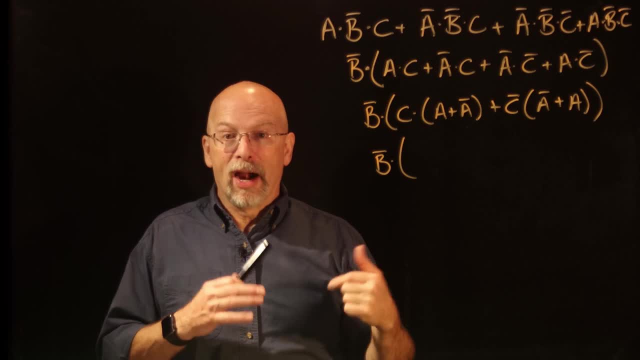 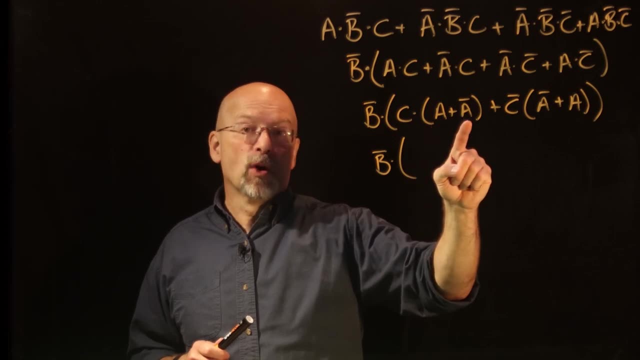 this product, pull it out and get A or A bar anded with C or C bar, But that's not what I'm going to do. What I'm going to do instead is see I've got something being ORed with its inverse. What happens when you OR something with its? 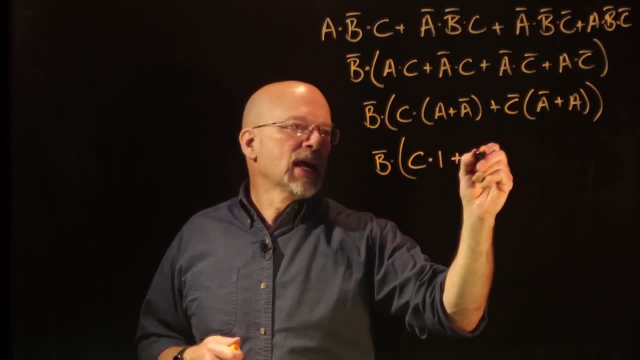 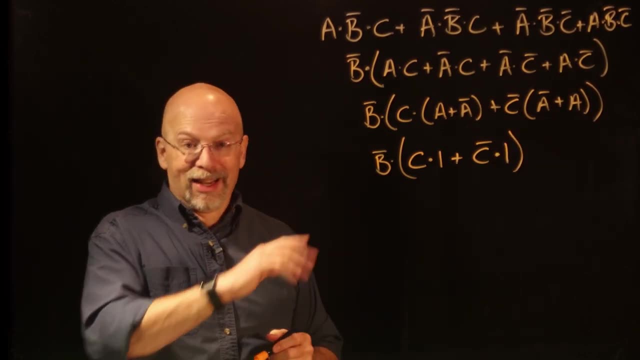 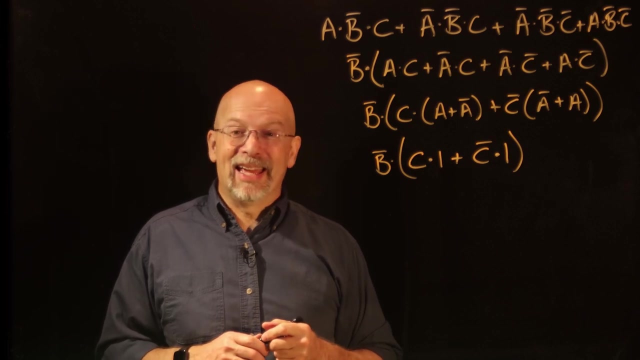 inverse, You get one Again here. I have something ORed with its inverse. I get one. all right, Now I have a glaring red flag. right, There's a constant that has showed up here. This constant, well, anything anded with one, Always itself. So 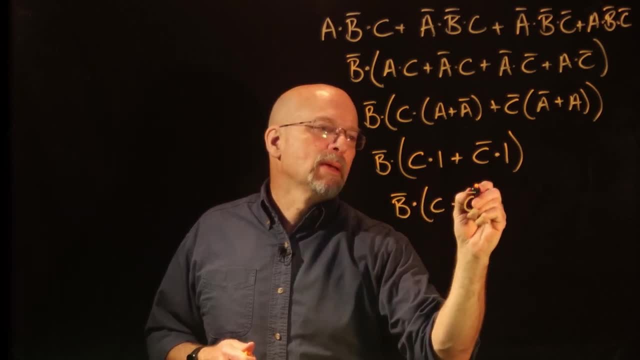 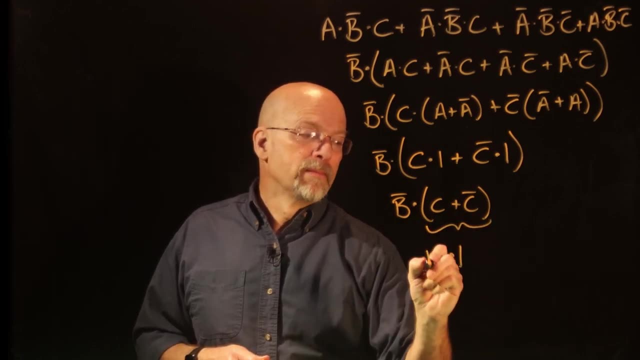 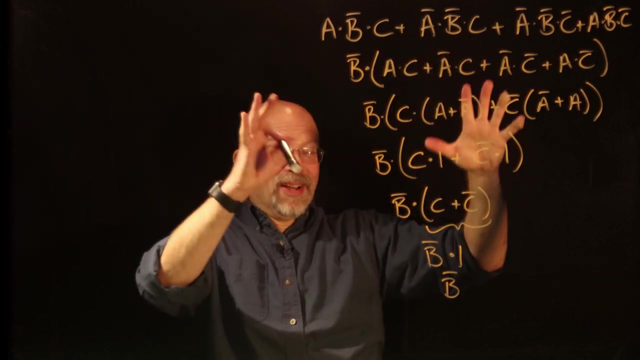 this becomes B bar anded with C or C bar. And then we once again have something being ORed with its inverse. That becomes one, This becomes B bar anded with one, That's just B bar. And so the final simplification, wow, the final simplification I have started out with. 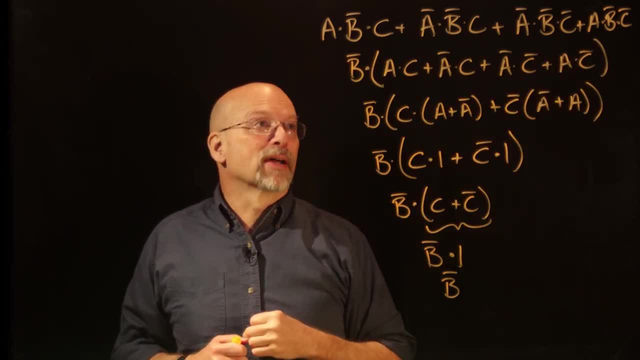 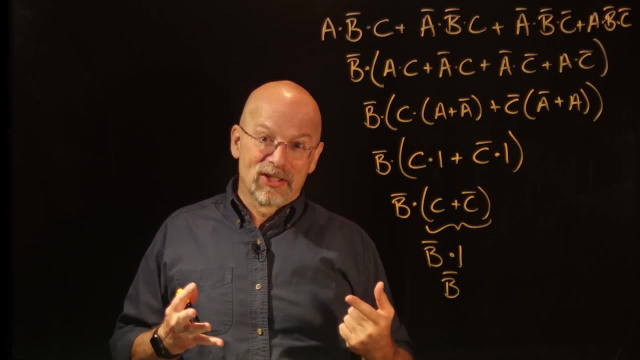 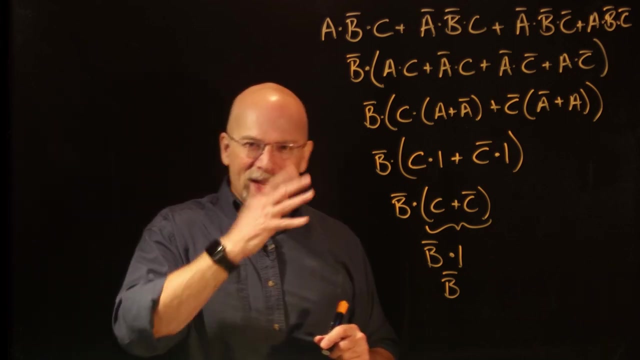 one, two, three, four, three input products ORed together with one, four input OR gate. That's a lot of gates. In the end just an inverter That all can be taken care of with an inverter. Now there's something else to kinda see here, And if you're familiar with this idea of ones, 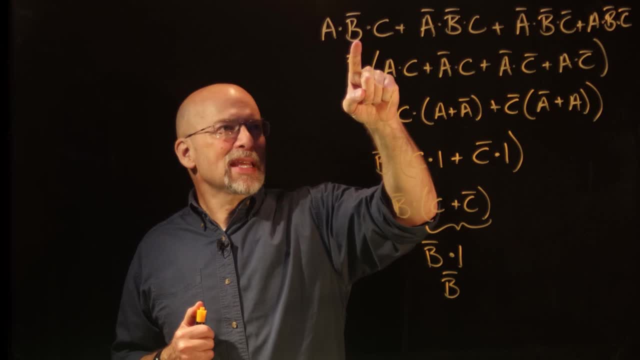 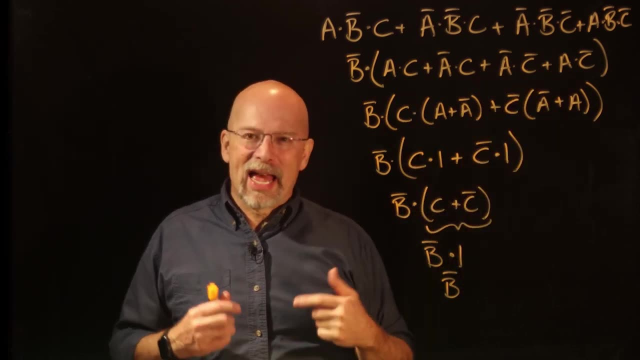 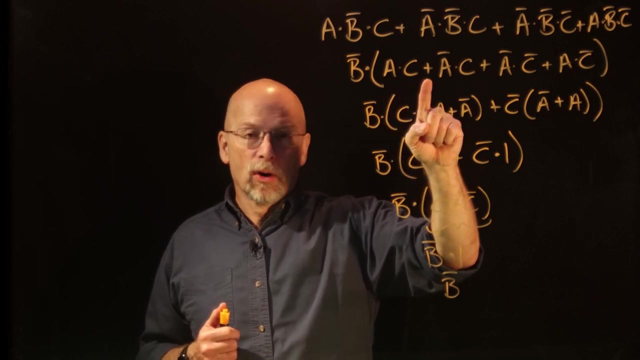 and zeros and the patterns of ones and zeros. you'll see that, yes, once we get to this second step here. this inside of the parentheses, has a unique pattern. What it's saying is: if A is a one and C is a one, or if A is a zero and C is a one, or if A is a zero and. 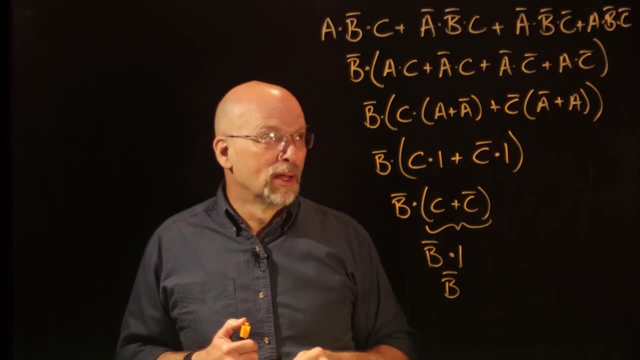 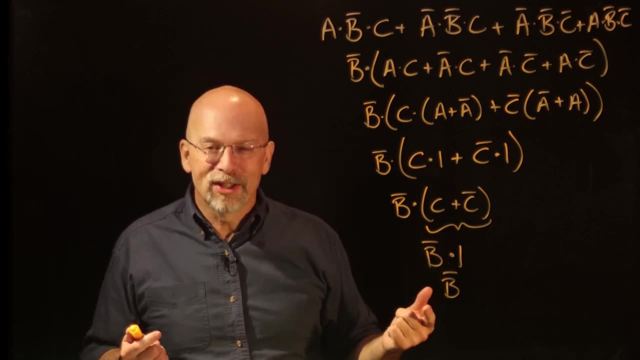 C is a zero, A is a 1 and C is a 0, then everything inside the parentheses is going to be 1.. Well, it turns out there's no other pattern of 1s and 0s that A and C could possibly take on, So therefore, 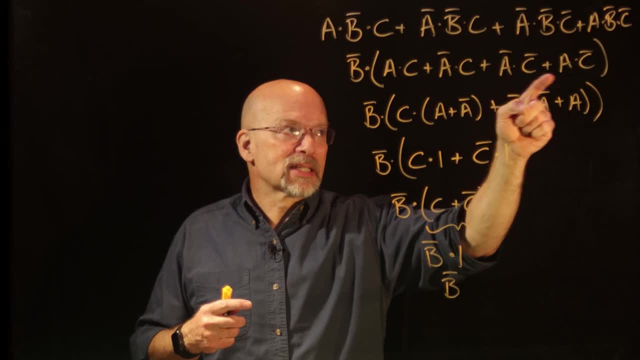 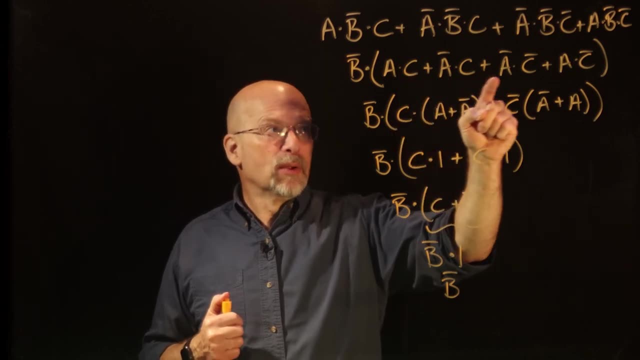 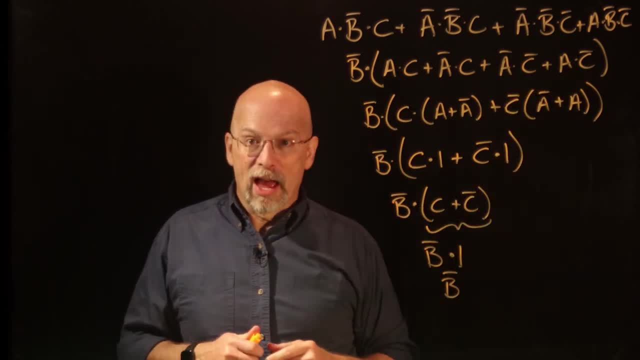 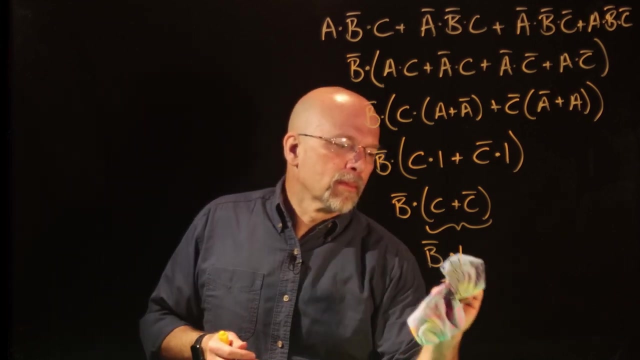 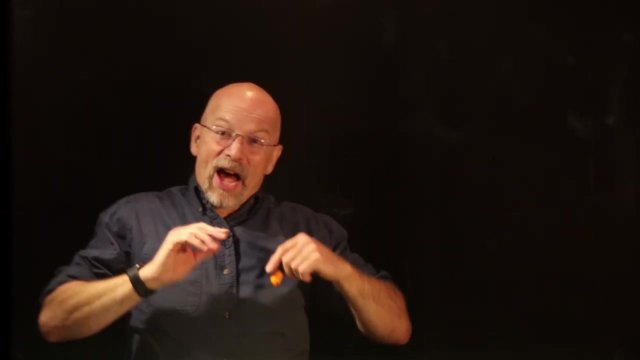 this OR inside of this 4-input OR gate. we're going to have a 1 there. We just did it using Boolean identities from here down, So there you go, Let's try one more. All right now, this next expression. well, it may not be as obvious as the previous one. 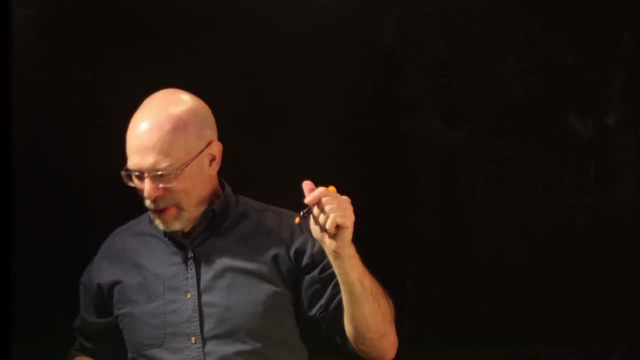 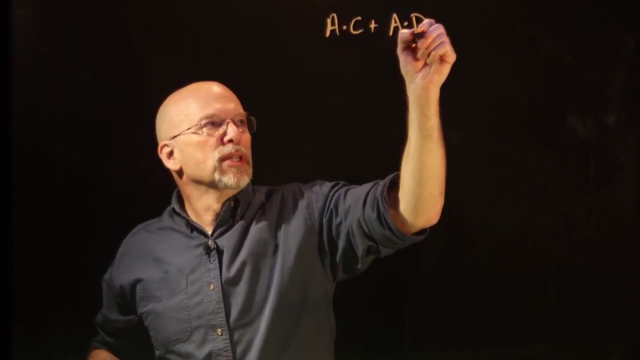 But let's go for it. I've written it down because I can't remember it. Let's see How about? A ANDed with C ORed with A. ANDed with D, ORed with A ANDed with C-bar and D-bar ORed with? 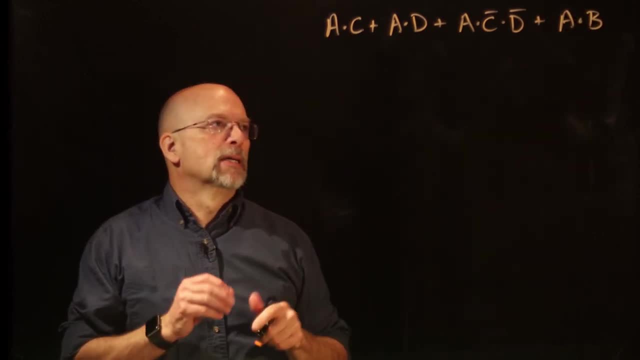 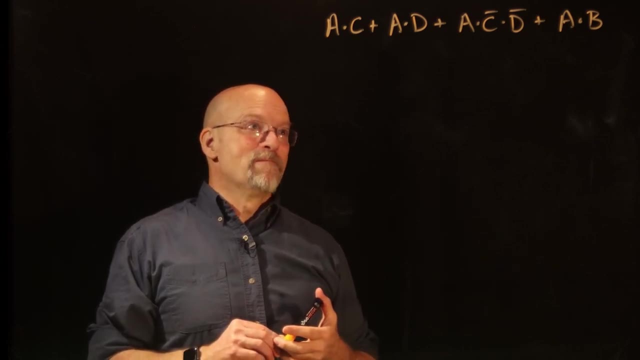 A ANDed with B. Wow, there really isn't any red flag showing up there, is there? Well, we do have an A in every one of those. So we have the four products that are going into a 4-input OR gate And A, and none of them are. 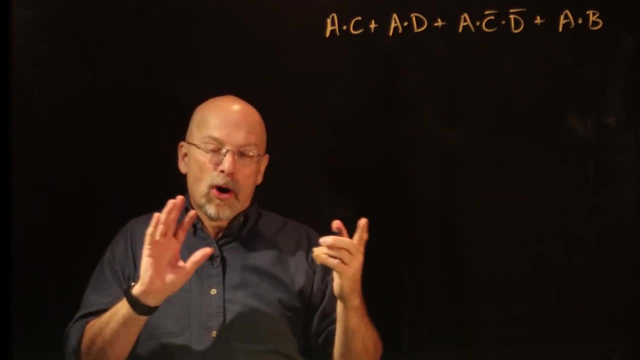 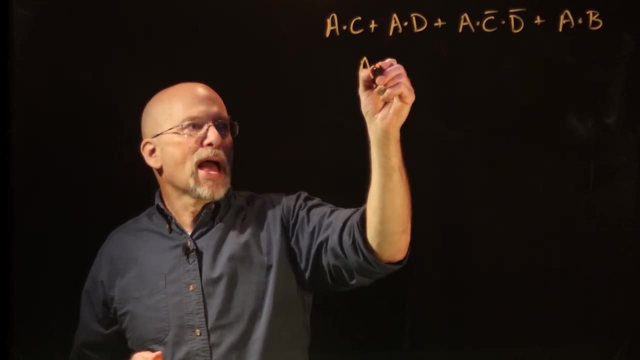 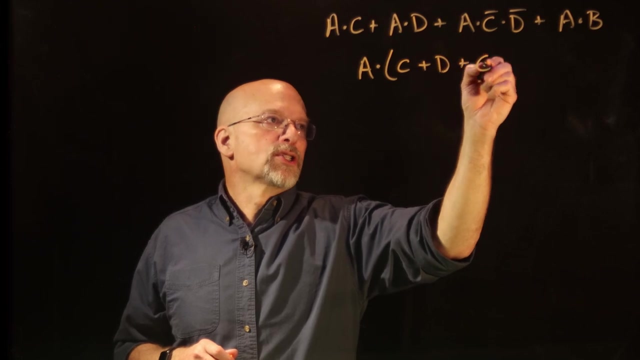 inverted, because if one of those were inverted, we can't pull out an A-bar with an A at the same time. All four of those A's don't have a bar over top of them, So I'm going to go ahead and pull out that A. Pulling out that A is going to give me C OR D or C-bar and D-bar OR B, right. 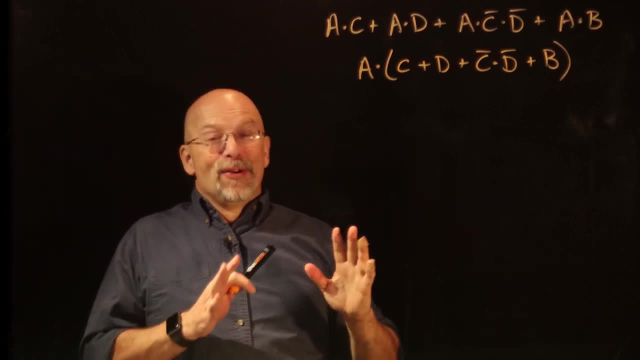 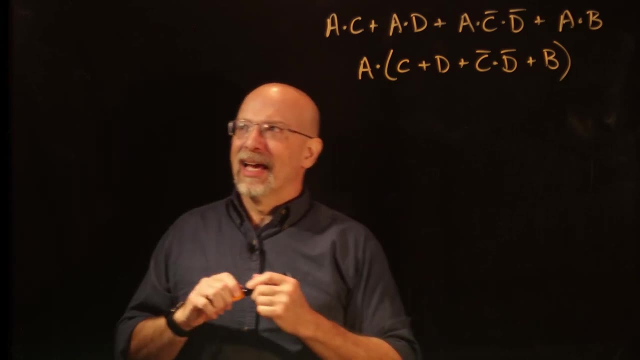 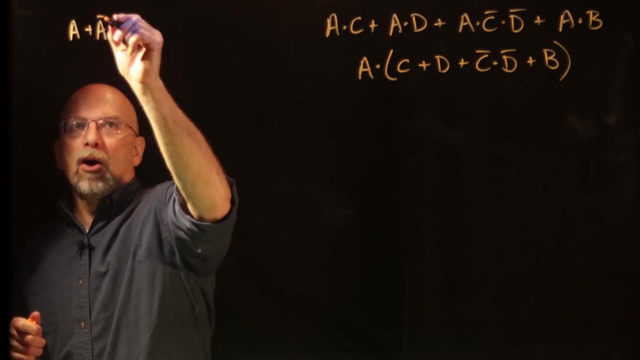 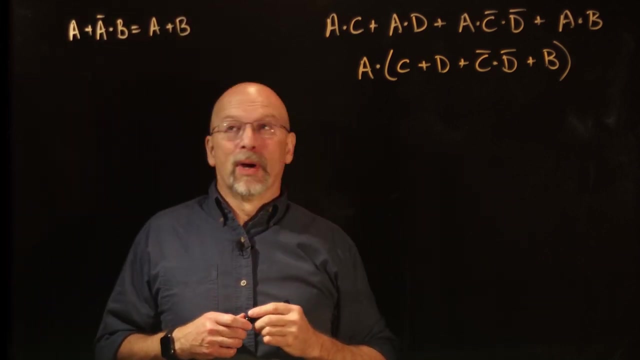 All right, Now there are a couple of ways we could do this. First of all, do you remember we had an expression or, excuse me, a property, that A ORed with A-bar B is equal to A OR B. Do you remember that one? Well, we have that kind of here, don't we? 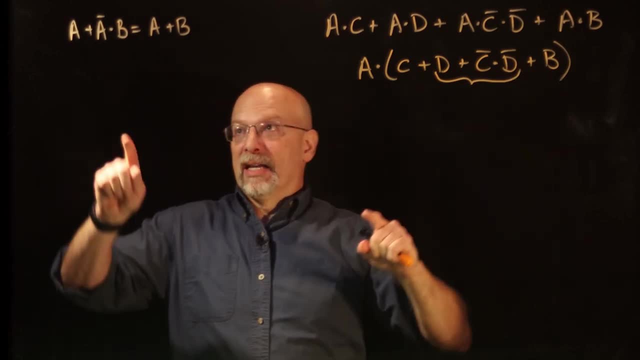 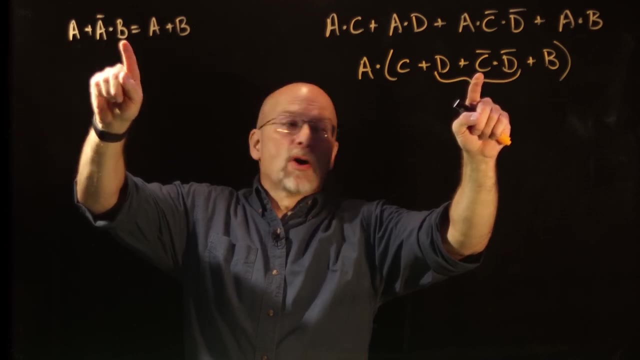 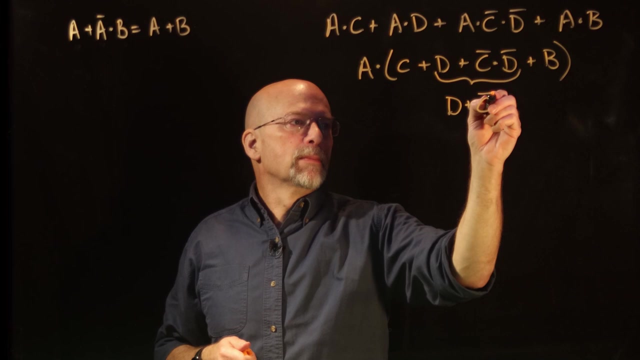 If I look at these two terms right here and I substitute D for A, which means D-bar is substituted for A-bar, and then C-bar is substituted for B, this guy is actually equal to D OR C-bar, So those two products and D really is a product. it's just a product with only. 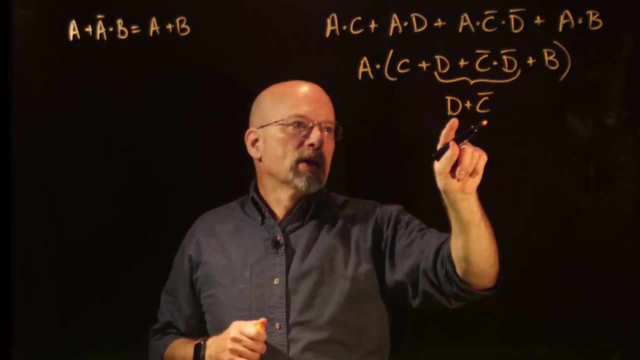 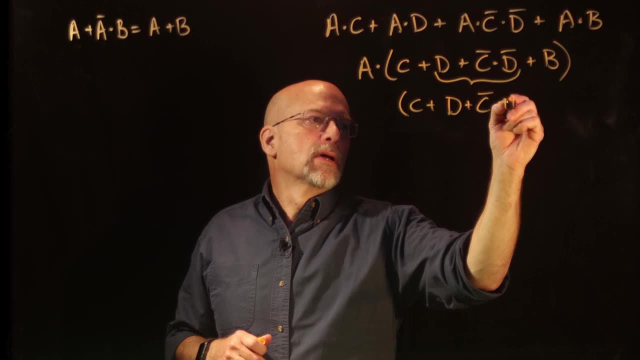 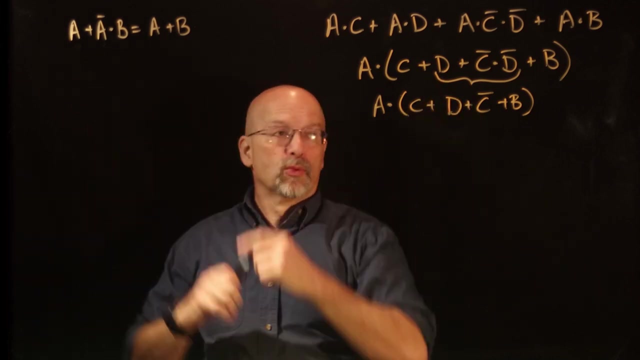 one input, D ORed with C-bar. D-bar is the same thing as D OR C-bar. Now let's bring down the rest of what's inside the parentheses and also bring down the A, so that now we've got this. moves to this once. we apply this rule right here. The other thing: 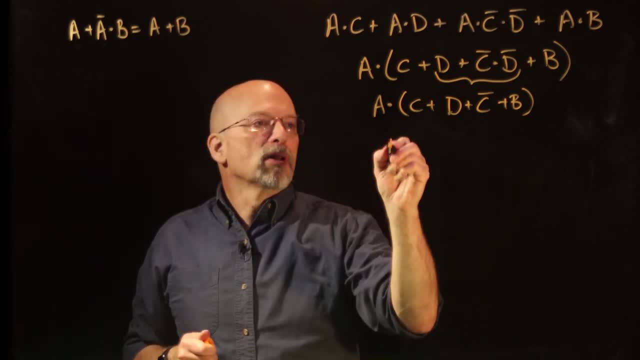 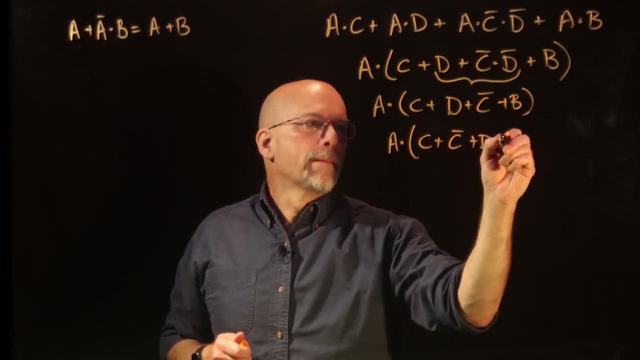 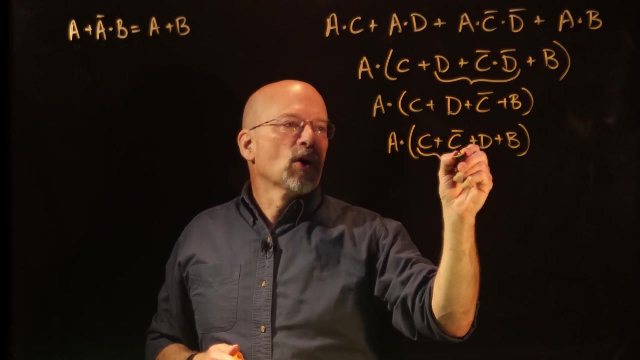 that we could do is use the commutative law, and the commutative law says: I can take these two terms and swap them around. All right, Hopefully you see the red flag at this point. We've got something ORed with its inverse. All right, Something ORed with its inverse. 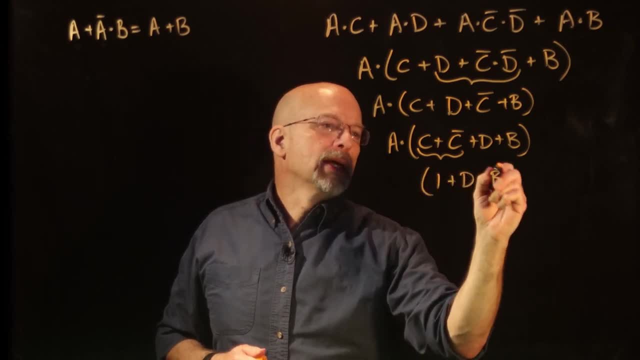 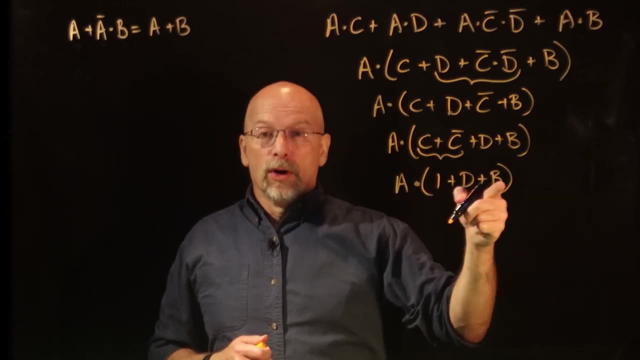 is always 1, so we get 1 OR D OR B. Of course, don't forget our ANDed with A. Anything ORed, excuse me, anything ORed with 1 is 1, right A, 1 goes into an OR gate. 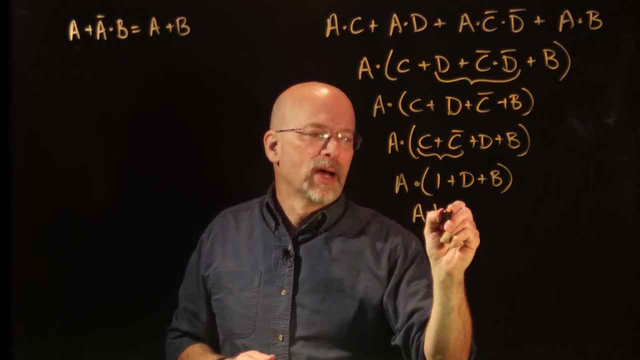 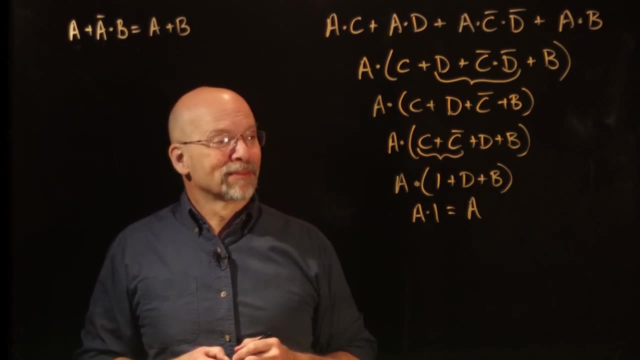 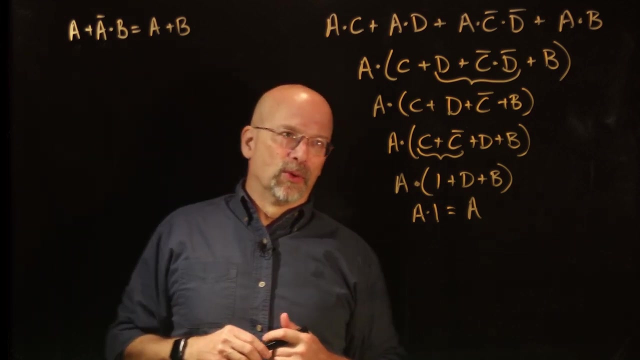 a 1 comes out of the OR gate, So we've got A AND 1, which is equal to A. All right, Well cool. There's another way to do this, though, and this other way is very different than the application of this rule. What I could do is start with this guy, In fact. 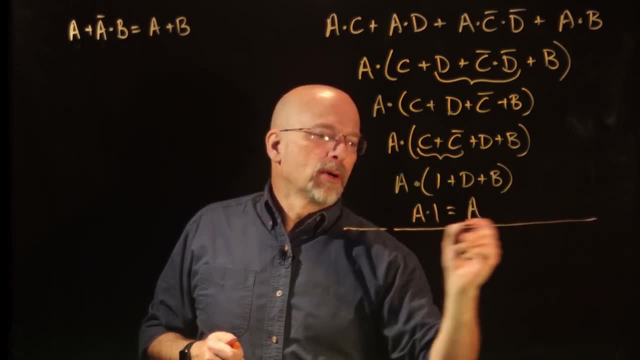 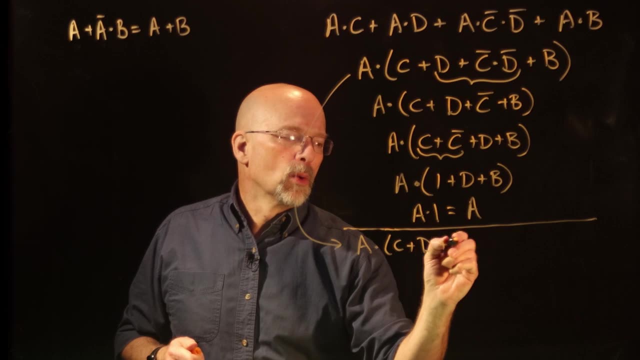 let me go ahead and bring this one down. I'm going to put a little line here. We're going to bring this guy back down here, so we'll have A ANDed with C OR D OR C-bar, D-bar OR B. Okay, 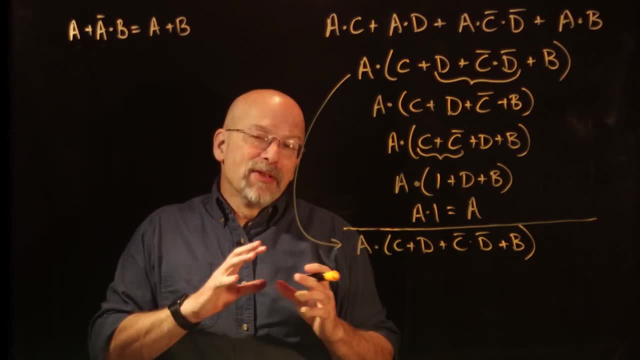 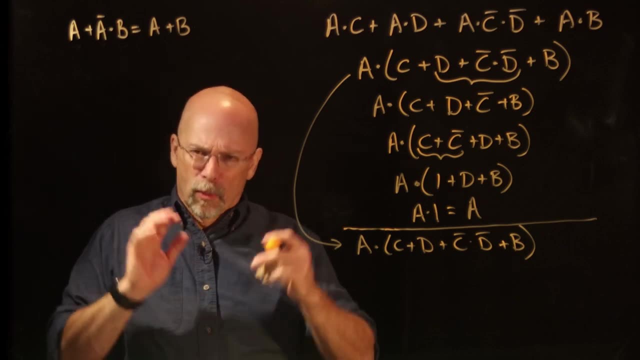 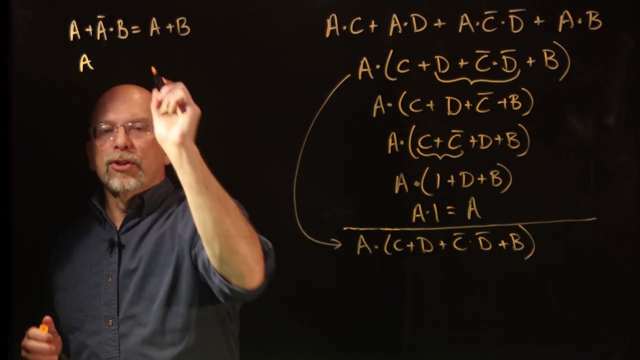 Now, this may not be obvious to somebody who is just starting out in simplification, but it turns out we have an application of De Morgan's theorem, one of De Morgan's theorem's forms in this expression. Remember, what I've got is there were two versions. 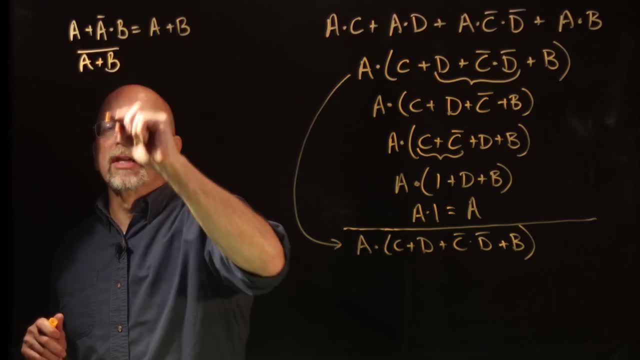 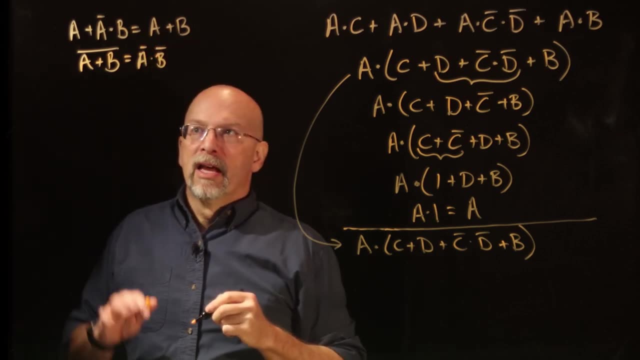 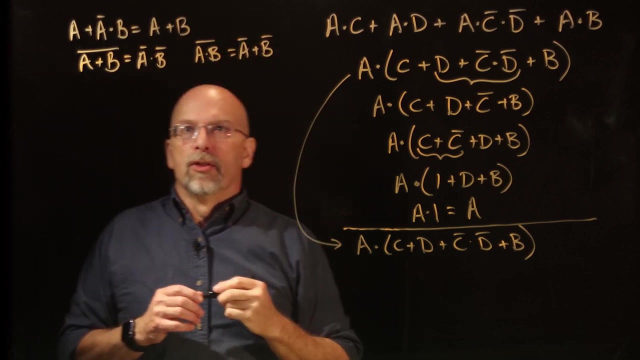 of De Morgan's theorem. One said: A OR B, the inverse of A OR B is equal to A-bar ANDed with B-bar, All right. The other version said that the inverse of A AND B is equal to A-bar OR B-bar, The way. 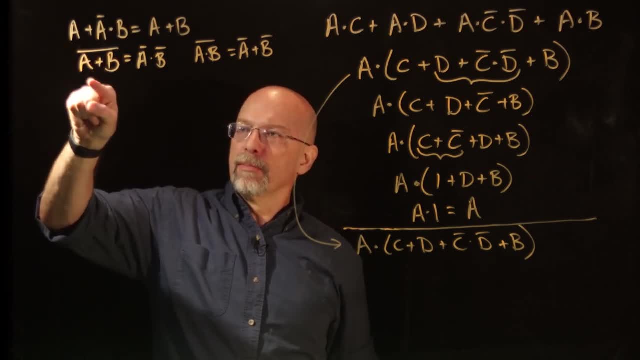 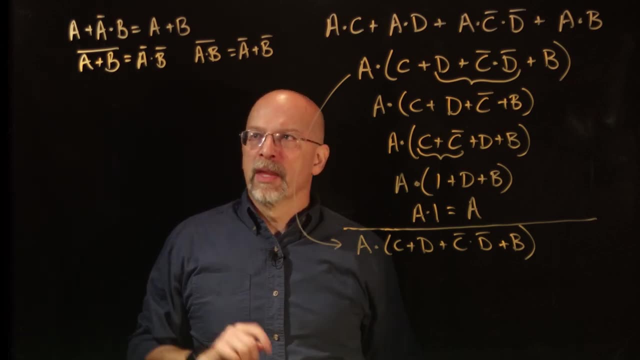 that worked was: I can distribution the bar to the inputs as long as I change the operation. I can distribute the bar to the inputs as long as I change the operation. Well, look at this guy. I could actually apply this backwards, right, The other way around, Instead of distributing. 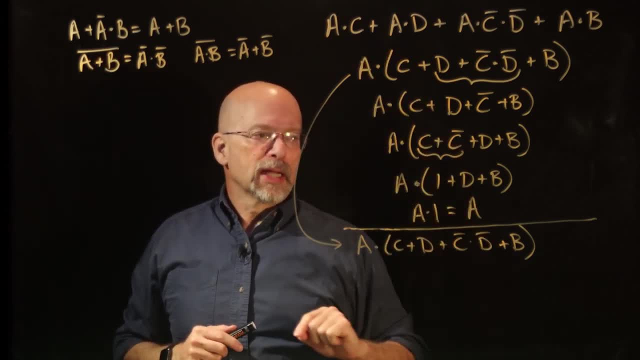 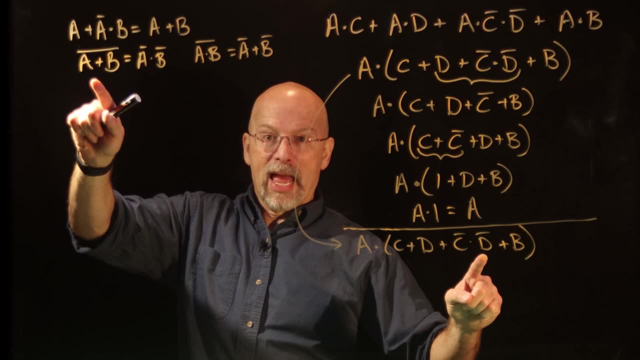 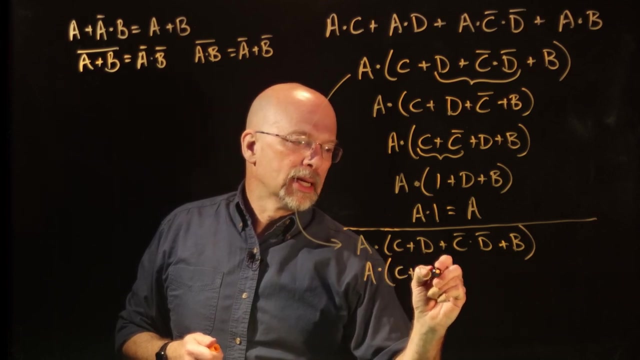 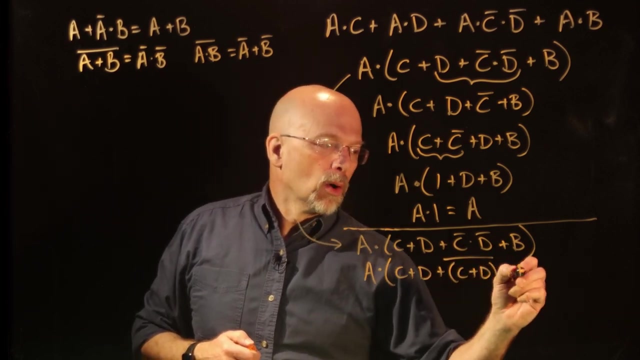 I could pull the bar out. Look at this C-bar AND D-bar: C-bar AND D-bar. That looks like form, right. If I go backwards and make it A or B inverted, I get A anded with C or D or'd with C or D inverse, the inverse of C or D or B. All right, Now the commutative law says I: 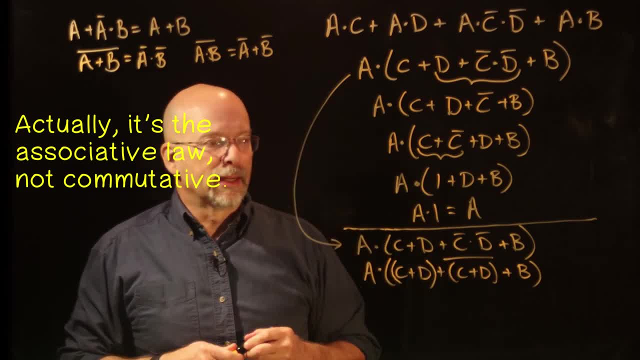 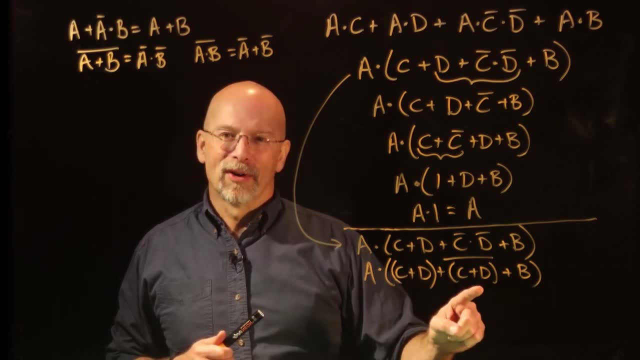 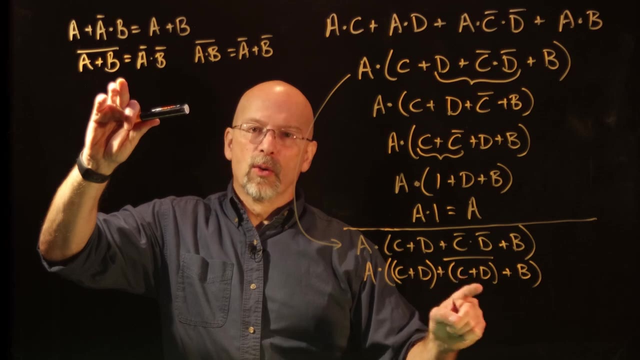 could also just simply put parentheses around C or D And look at this One step earlier. we got something or'd with its inverse. This is just by an application of DeMorgan's theorem. I've got something or'd with its inverse. What happens when I or something with its inverse? 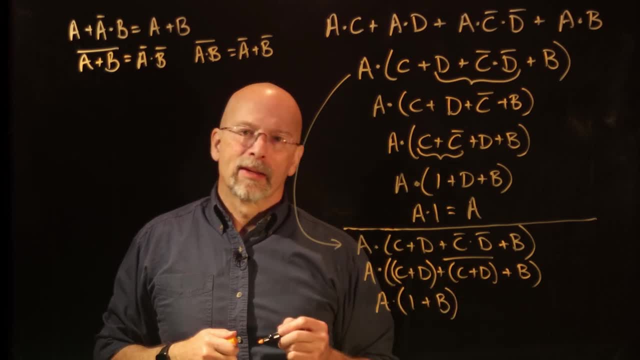 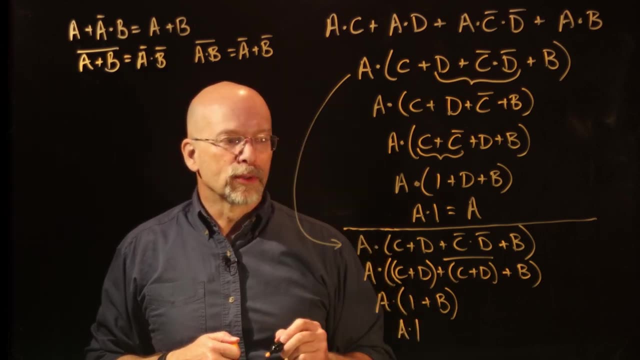 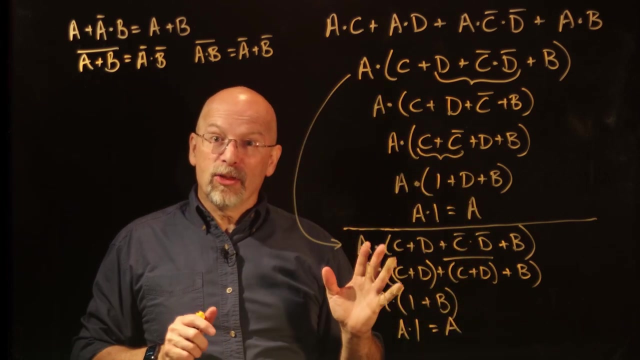 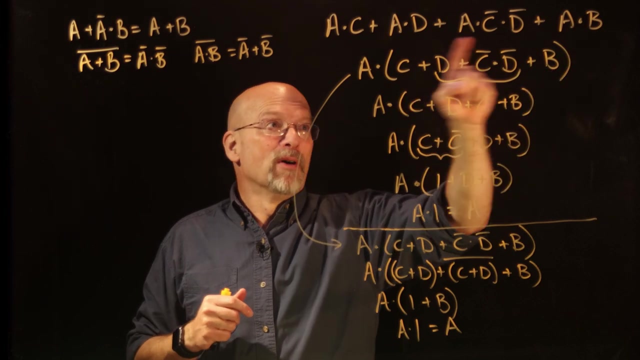 That's going to be equal to one. What happens when I or one with something That equals one which equals just A? And so our final result, no matter what path we took, is simply that: Gosh, once again I've got four products and one four-input or gate combining all. 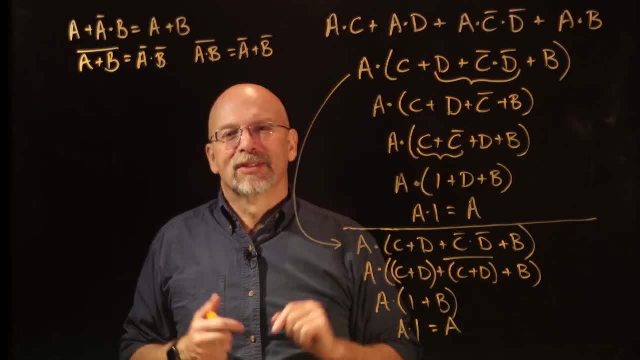 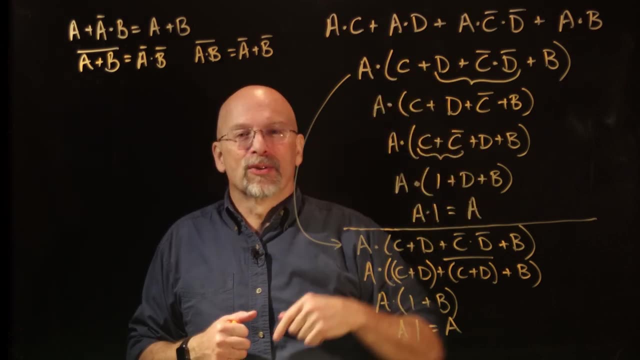 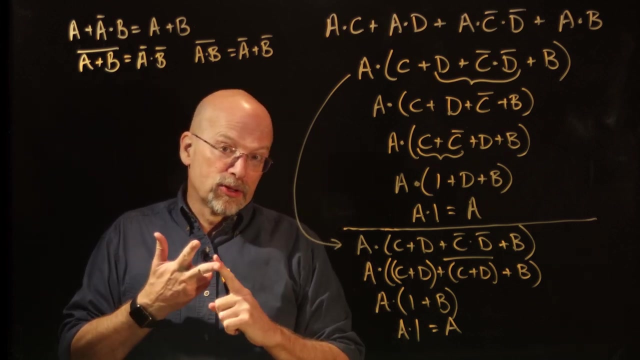 of these signals together. All of that filtered its way down to just a wire. Just A is driving whatever. As long as A is true what we're looking for, this expression right here, it's true too. All right, Hopefully. the three examples from the last lesson and the two examples from this lesson. 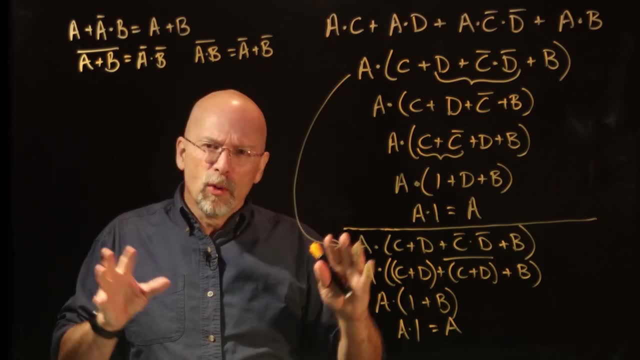 will give you an idea of how to slowly but surely move your way forward through simplification of these Boolean expressions.